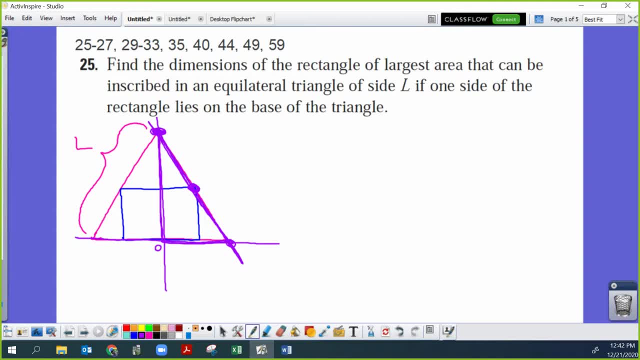 ratios of those, because it's a special right triangle. In fact, we're going to use that knowledge whether we do the coordinate system or not. I'm actually going to ditch the coordinate system here. You could do it that way. If you found the coordinates of these points, you could. 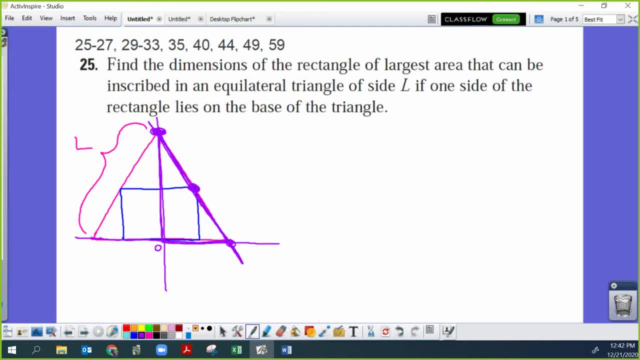 do slope and then write slope intercept form and use it that way. However, I kind of think this one might be easier to just again kind of use the similar triangles: the 30,, 60,, 90s. So we have one. 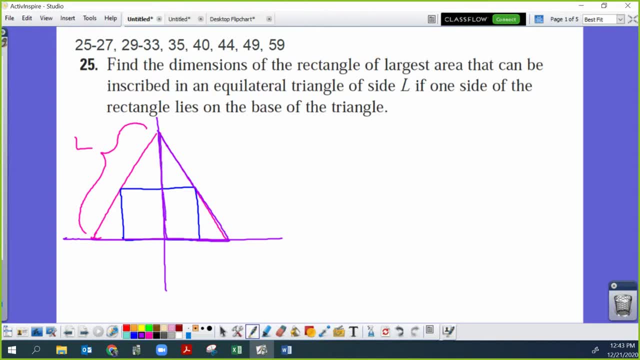 right there. And then I know right, You thought you're done with geometry. Calculus is where it all comes together, guys, And you know what, Like the 30,, 60,, 90 triangles. you did that last year, You've. 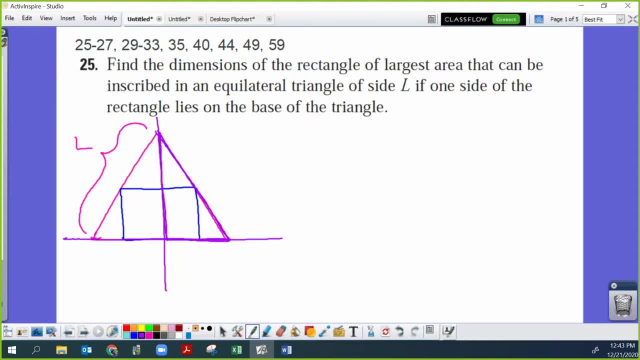 done it every year, right, Because it shows up in trig, so much I know. So where else do I have? what can I do to relate that triangle to like something that helps me with the dimensions of that rectangle? Yeah, I need. so I've got this big 30,, 60, 90 triangle, but I might need a different one so that. 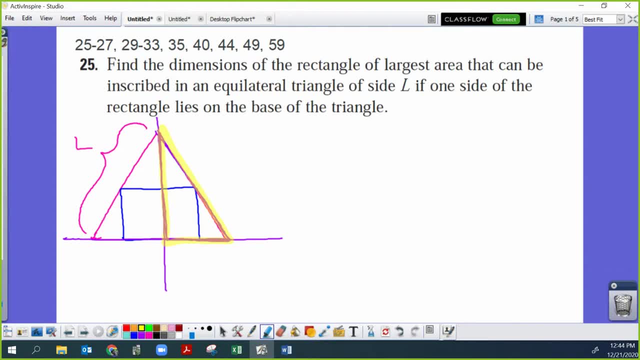 I can tie it to the rectangle more directly. Yeah, so we got a couple other ones there. We got, we got this one and you could use that one Or even better, I think easier would be okay, That one. Oh, okay, Now it might be tempting. I just want to caution here. I actually did this. I. 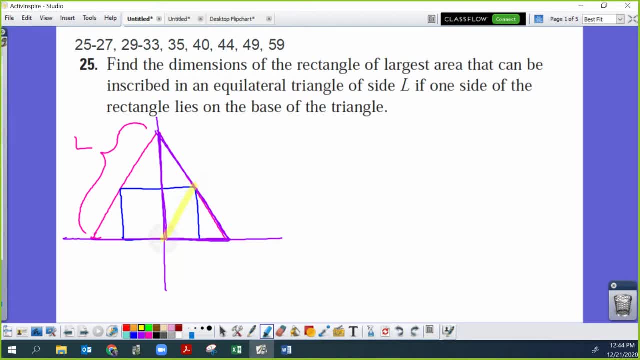 did this in first period today, I made a total noob mistake. I was like, oh, what about this triangle? That's probably similar to the big triangle And it's not necessarily. It's probably not Like it could be at one iteration. But just to make my point, if you did the rectangle a bit, 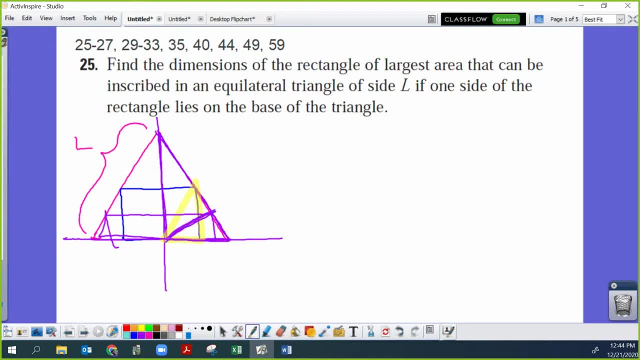 lower here you can see that that triangle would very much not be a 30,, 60,, 90. Or if it is, it'd be like the other way And that'll it'll only be at one spot also. So so it's not that one, All right, So we want this one, That's. 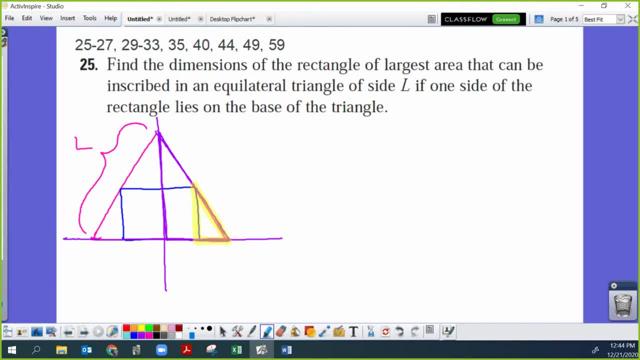 also does everybody see that that has to be similar to that bigger purple one. It's got a shared base angle and they both have a right angle. So it's also a 30,, 60,, 90. And if I, if I call this height here of the rectangle Y and then if I call this like right here, X. 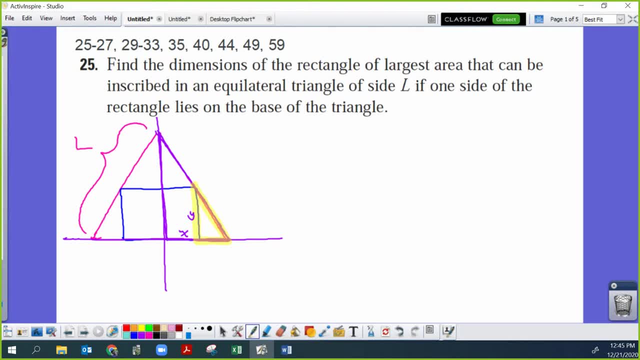 then my rectangle's area is going to be: what, No, Oh, what, Yeah, Yeah, Cause the whole base will be two X, right? So this is my primary equation, right, And we're like, we got our primary equation. The problem with it as written is that it has 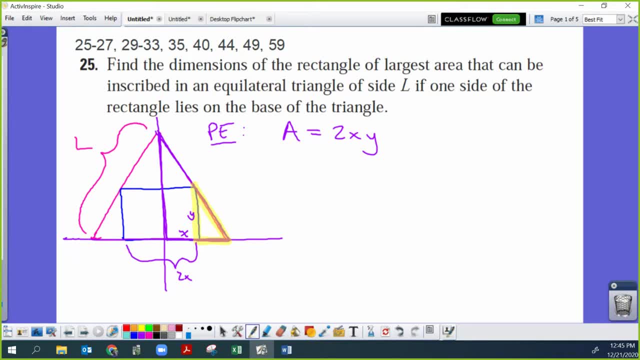 two variables. in it, right It's a in terms of both X and Y. So what we're trying to do is relate X to Y, probably using L, which, remember, is a constant, So that we can substitute in for one of them. 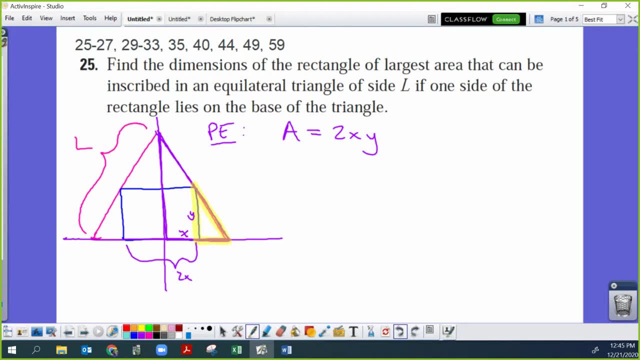 and have one variable, A in terms of one variable. So how do I do that? How long is that? That is 1 1⁄2.. Oh, 1 1⁄2 of the side of the triangle. Yes, that is 1 1⁄2.. 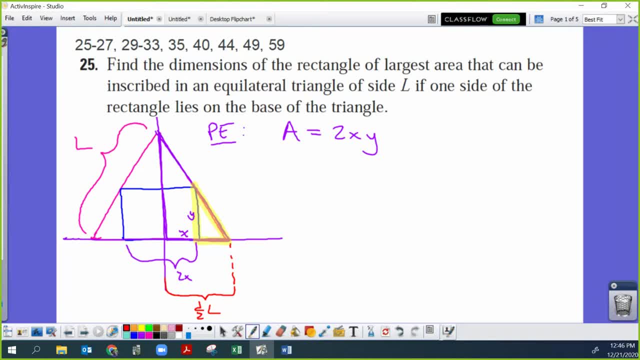 That's weird, Yep. And so what is that? One half L minus X? Yeah, it looked like Kenny was doing something right over here. That's good, Yeah. So then what's the relationship between one half L minus X and Y? 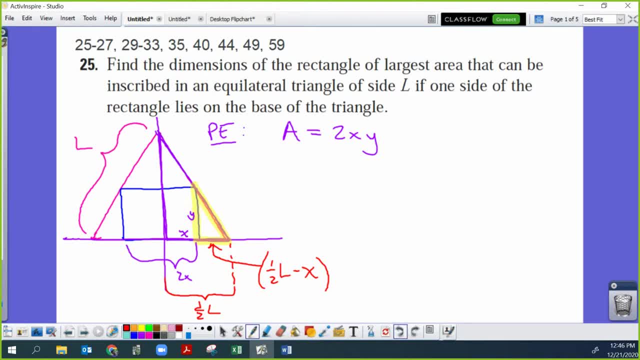 Given that that is a 30-60-90 triangle highlighted in yellow. So I would say it's actually the X, or sorry, the one half L minus X. L minus X times the square root of 3 is going to equal the Y. Does that make sense?